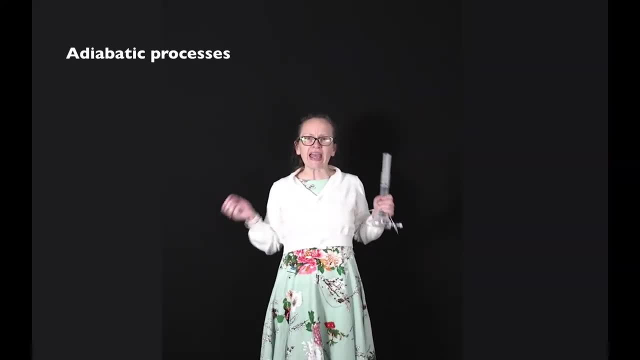 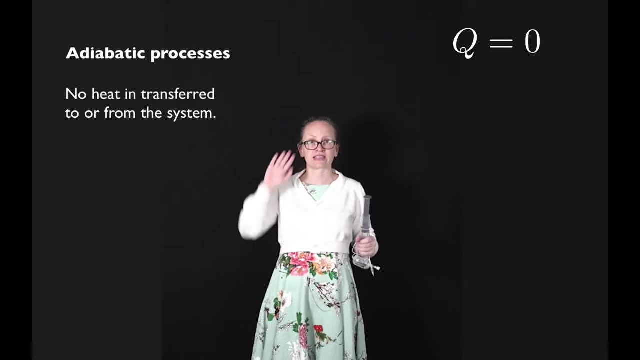 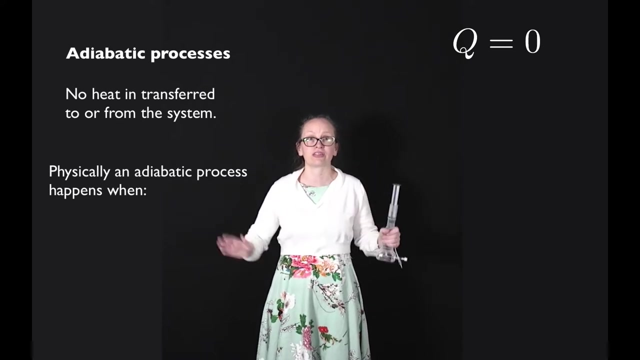 We're now going to consider adiabatic processes. So adiabatic processes are processes in which no heat is transferred. So as an equation we can say: well, Q is equal to zero. Now, physically. there's two ways that we can obtain an adiabatic process. One way is to use an insulated container such as a thermos. 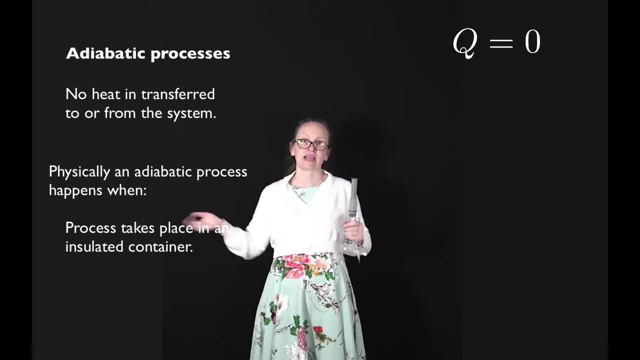 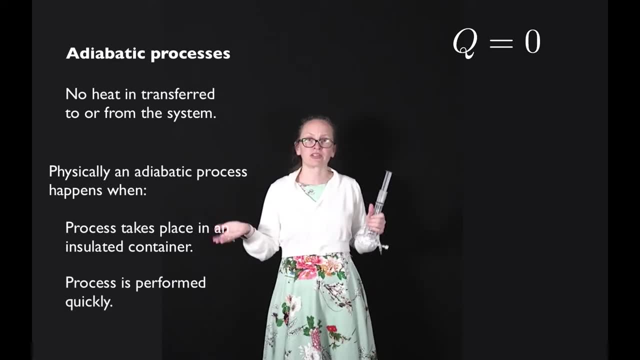 If heat can't transfer through the walls of the container, then there is no heat transferred to that system. Another way to do it is to perform the process quickly. So, for example, if I compress this gas very quickly, then that's an adiabatic process, because it takes time for heat to transfer. 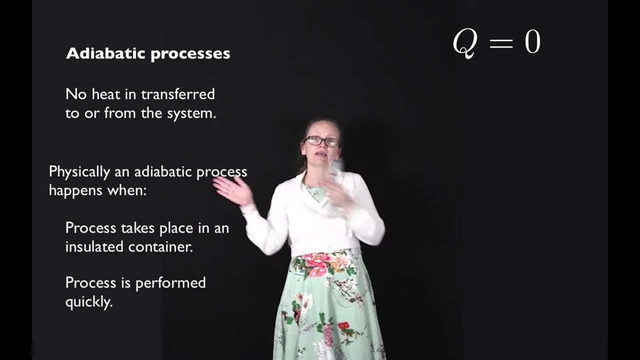 Heat transfers from the hotter body to the colder body, but it does so over a period of time, So doing it quickly means that no heat is transferred. So our first law of thermodynamics: the change in internal energy is equal to Q plus zero. 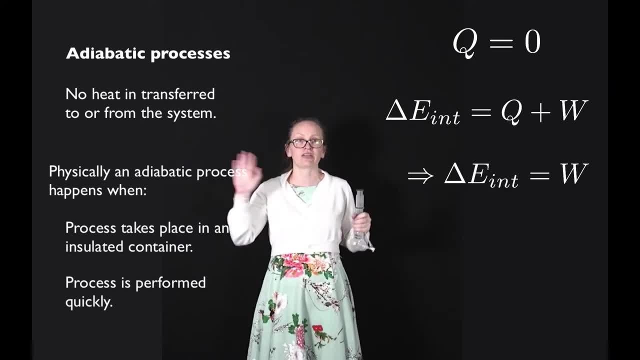 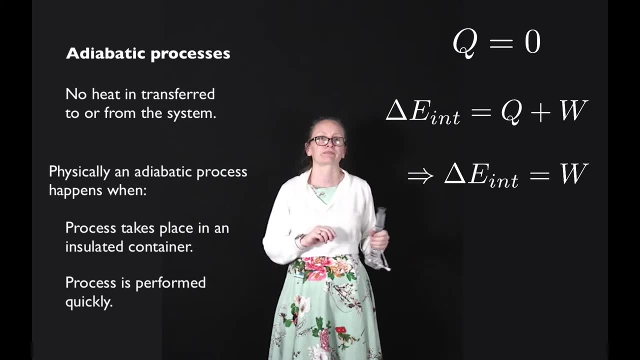 So the change in internal energy is equal to W. for an adiabatic process This becomes that the change in internal energy is equal to W the work done on the system, because Q is equal to zero. Now a really boring example of an adiabatic process. 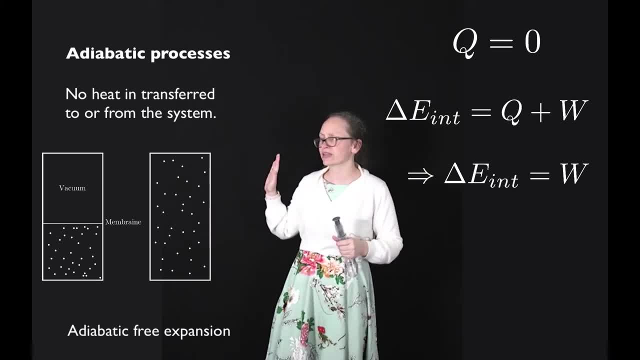 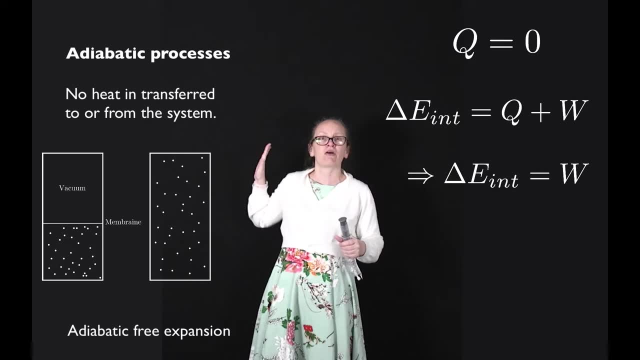 is adiabatic free expansion. So imagine that we had a cylinder and we compressed all the gas molecules into the lower half of the cylinder and topped it off with a cylinder. So this is a really, really thin membrane. Now if you imagine very gently breaking that membrane, 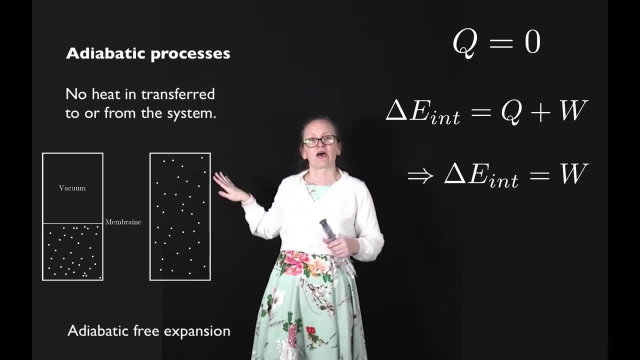 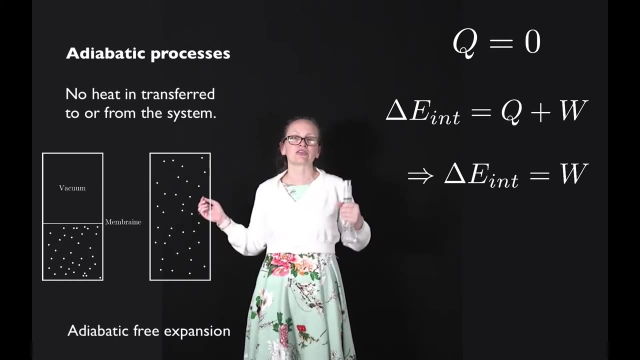 so we're not doing any work in this process, we're just very, very gently removing the membrane. in that case, the gas molecules, which were confined to the lower half of the cylinder, will be free to expand into the upper half of the cylinder as well, And so in this case there is no